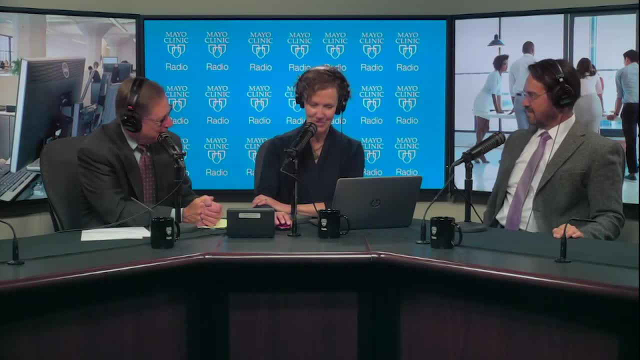 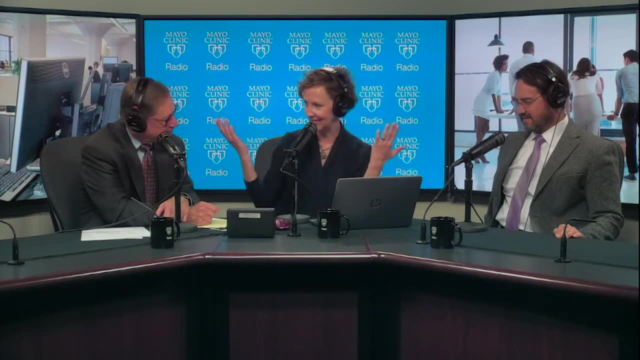 Well, that's true, That's over a year. That's a lot Over time. Tell us more. Those missing calories could lead to a five-pound weight loss each year. And if the problem is you end up gaining 10 pounds a year, you know, just do the math. 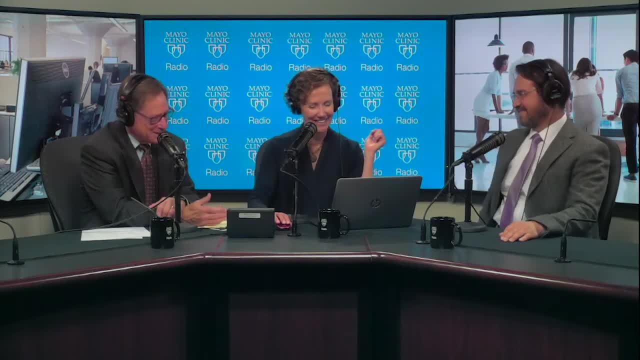 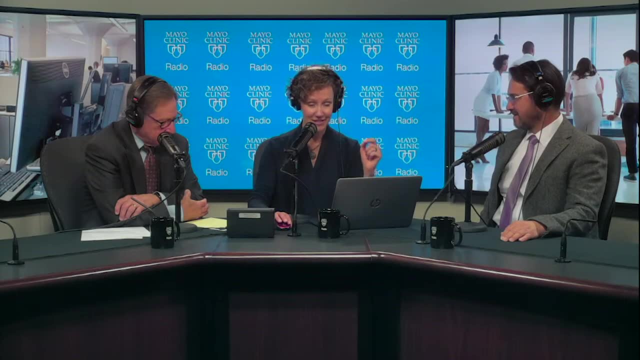 Don't make me do any more math. Exactly, It's like just a little bit of exercise every day makes a huge difference. Here to discuss is the lead author of the study, Dr Francisco Lopez-Jimenez, Division Chair of Preventive Cardiology at Mayo Clinic and also Research Director of the Dan. 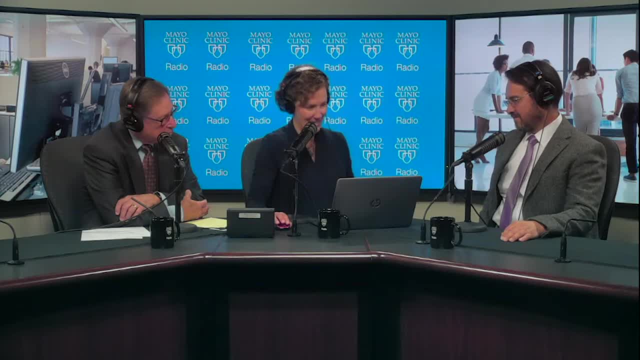 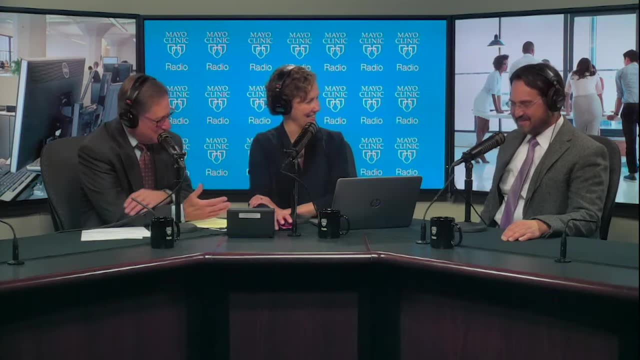 Abraham Healthy Living Center. Welcome back to the program, Dr Lopez-Jimenez. Hi, thank you. Thank you for the invitation, Dr Lopez-Jimenez. good to have you. You wear a lot of hats, sounds like, But what we want to talk. 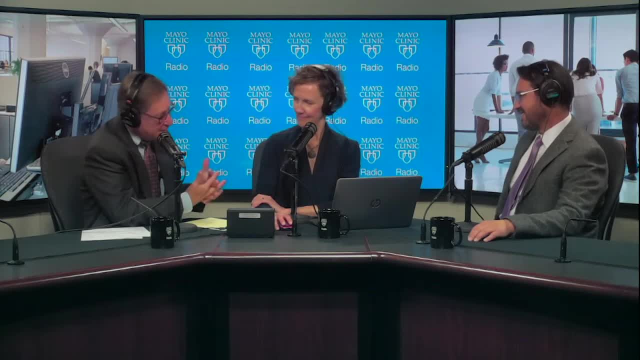 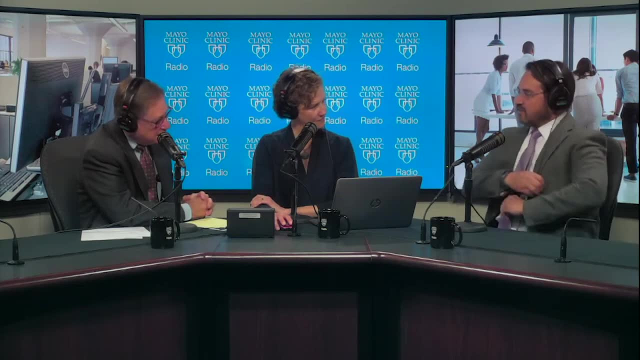 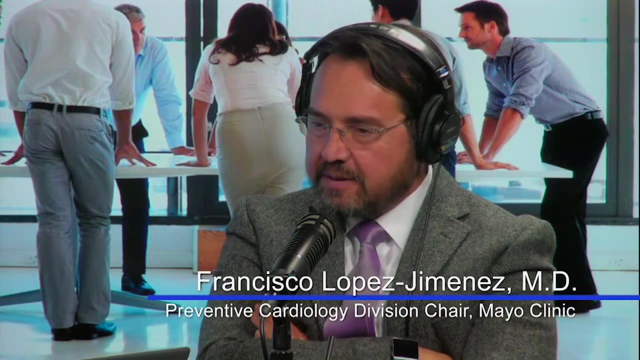 about today is sitting versus standing, And there is some pretty good evidence that standing at your desk instead of sitting does have some real health benefits. Yes, Well, one of the potential benefits is related to the caloric expenditure, as you mentioned, But we believe that the benefit might actually go beyond that. might also. 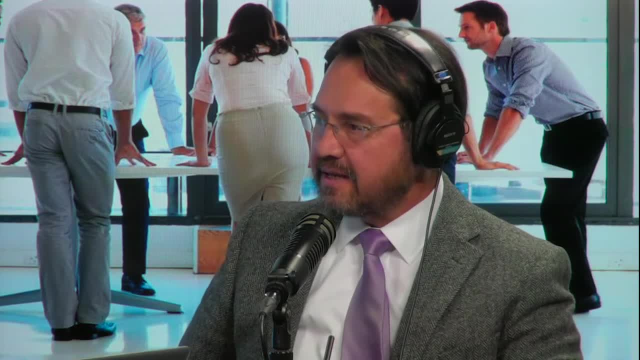 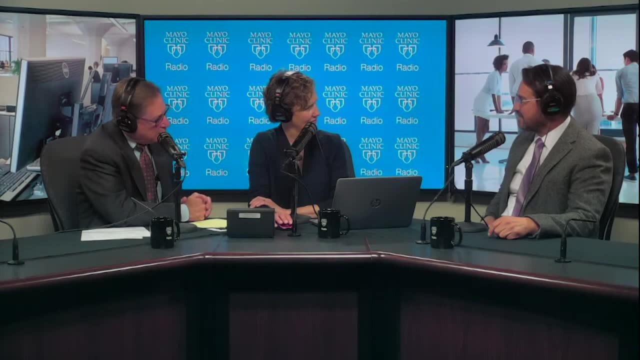 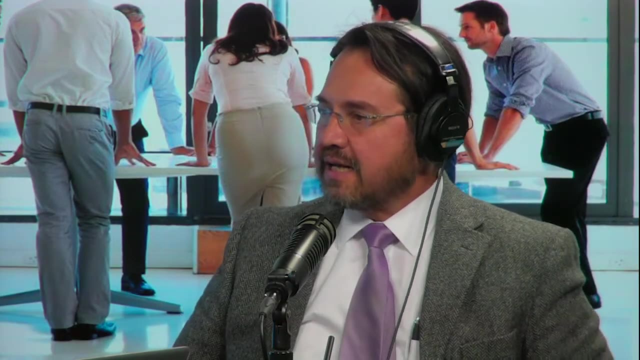 relate to the fact that there are more muscles activated And therefore there may be some benefits to the cardiovascular system. To the cardiovascular system, Yeah, Just by standing. Yeah, Well, you know, what we know is bad for health is sitting for too long. What is still? 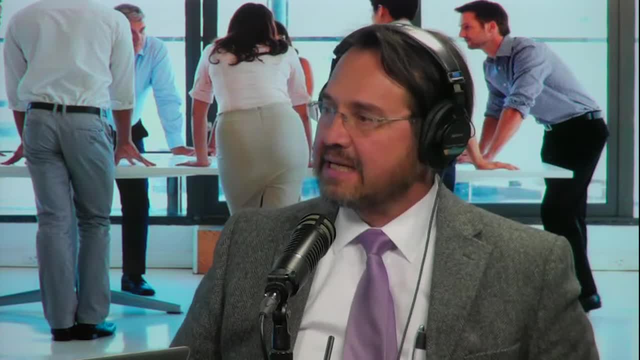 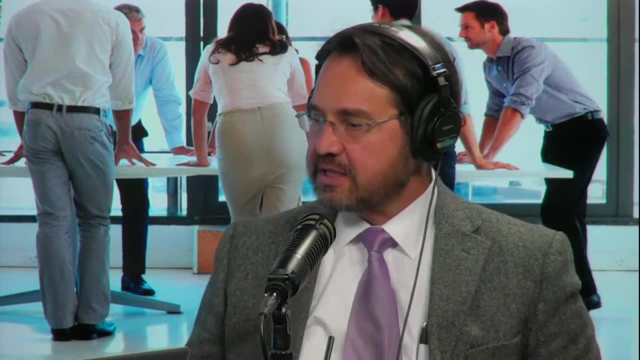 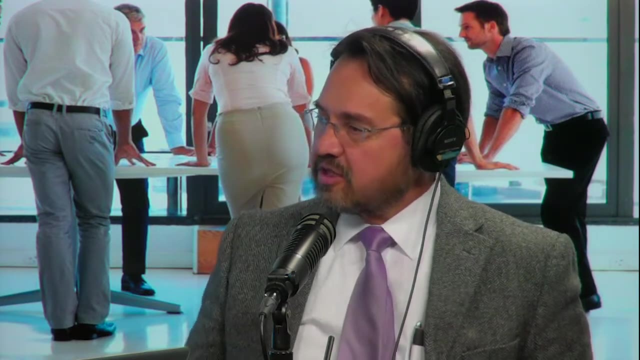 controversial is whether or not just standing will be good enough to avoid the consequences of sitting. Now this research essentially shows that there is some extra caloric expenditure during standing, which means that that is kind of half of what you do when you are walking. 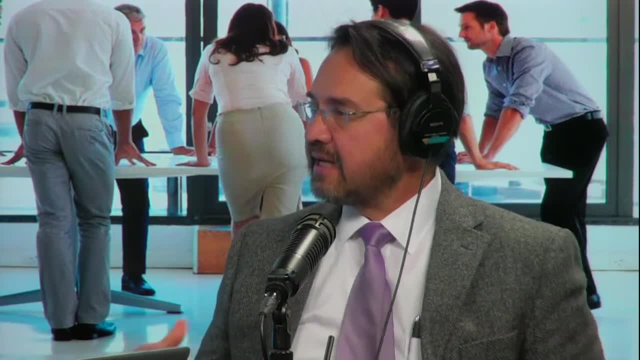 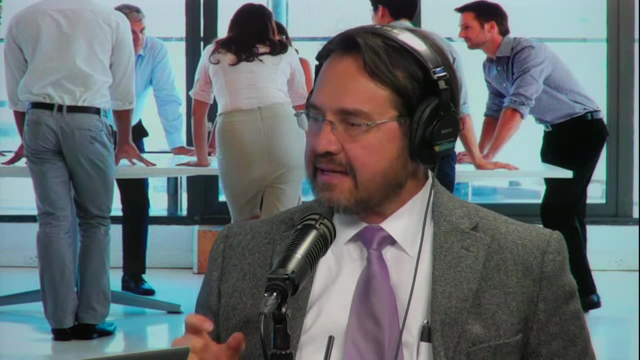 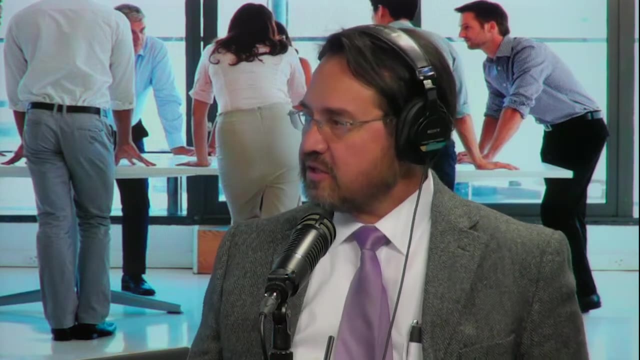 And if we believe that walking is good, then standing by itself might be certainly better than sitting. The secondary benefit with standing is that when you stand up it is much, much easier to do spontaneous activities. So it's not that you just stand, So it's easier just to. 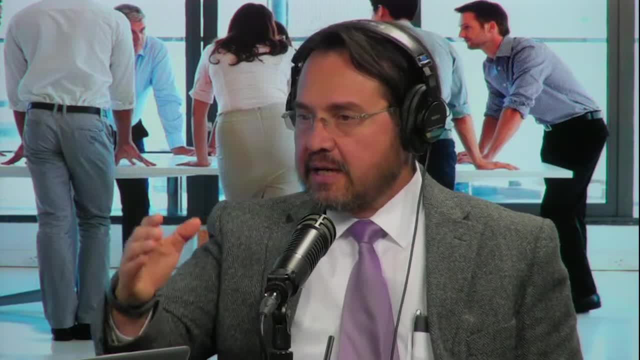 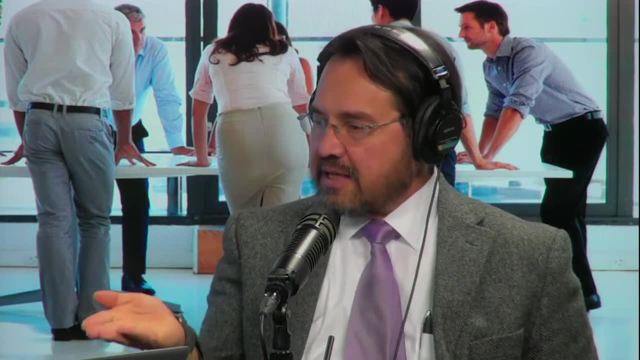 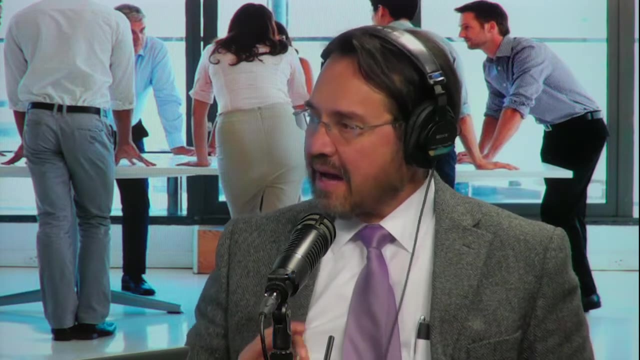 move from your office to the trash can and to the next door's office, moving around the office. So those experiments in our study were done just standing. So what's the simplest thing? But the benefit might actually go beyond that because you move more. 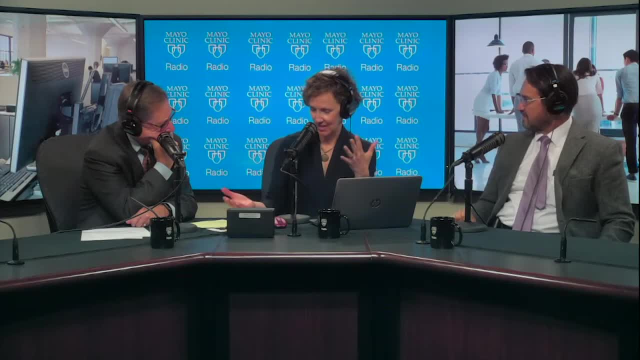 You know what, Now that you say that, so we put the, I put this show together at my house, in my office, And when I am standing I never thought about that, But when I am standing I've got, you know, like a balance ball and different things. 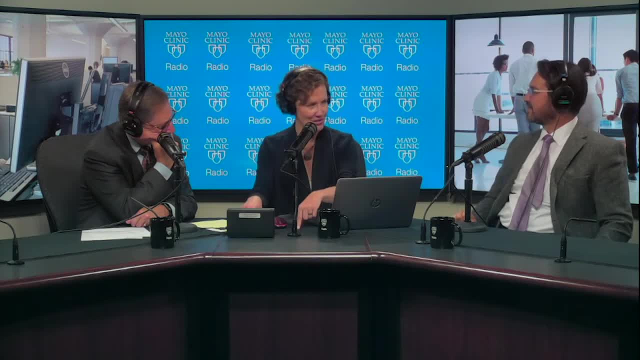 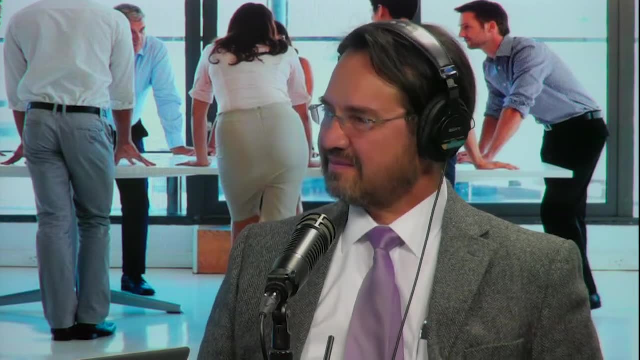 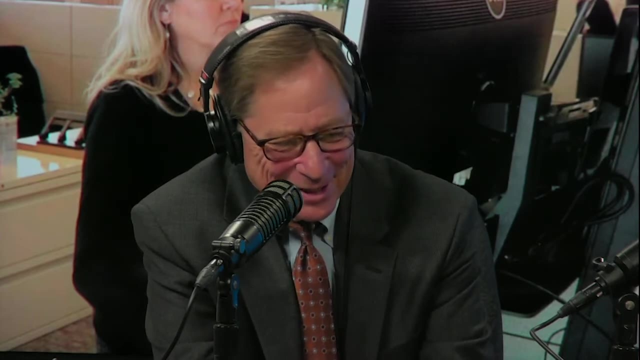 like that. When I'm standing I'm more likely to go over and do some of those exercise than when I'm sitting and editing the program. He must be right. I think he is. And you know, my wife got me one of those fancy watches. you know I won't tell what kind of watch it is, But you're trying. 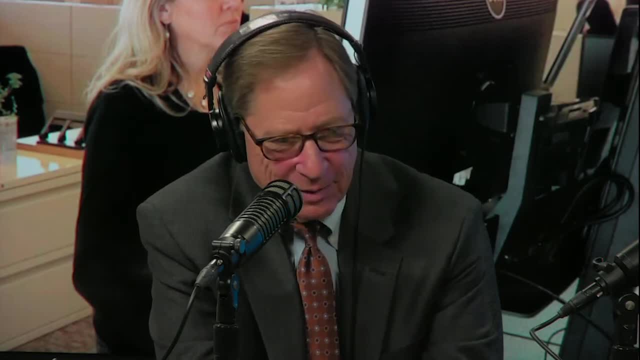 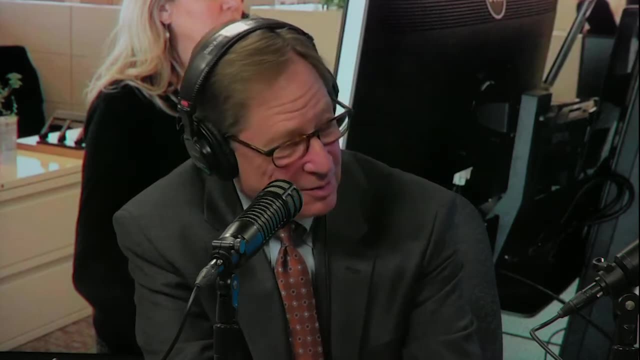 to figure out how to use. Well, no, and I didn't think that I would really needed one, but now I wouldn't give it up. And every once in a while, if I'm sitting at my desk, it will buzz on my wrist and it says: stand up. 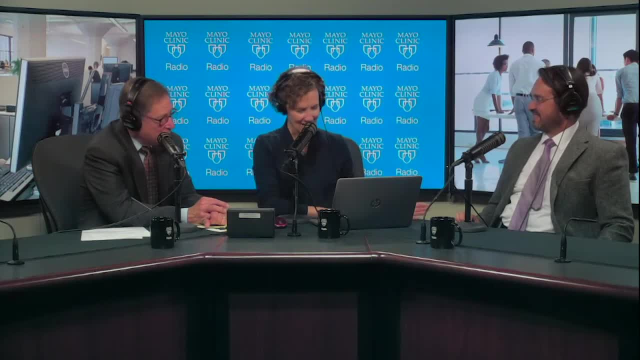 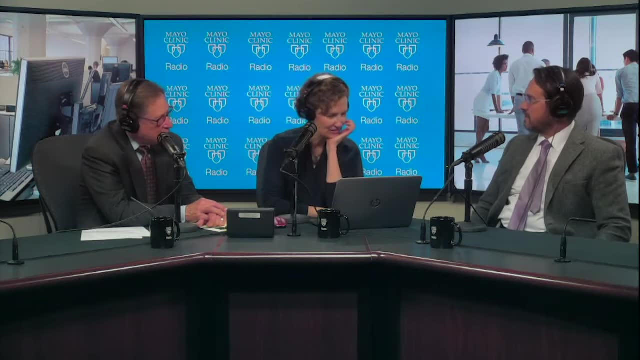 get up and move. Yeah, Interesting. Yeah, I guess there must be something to it. How much time does the average American spend sitting each day? About seven to eight hours a day, And that's about six to seven hours or eight hours too much. 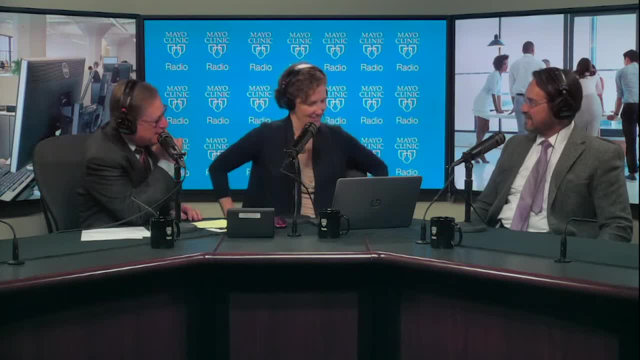 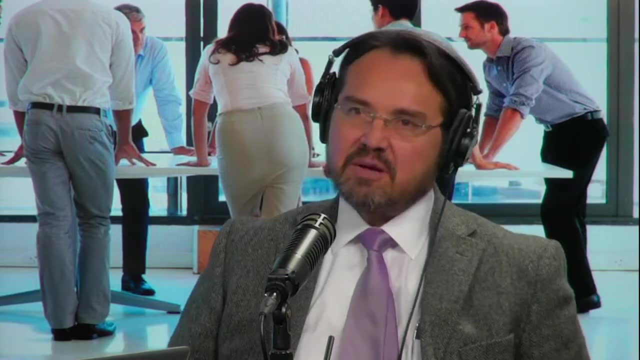 So you have a standing desk? I do, Yeah, Yeah. So Do you ever sit down or not? much for lunch I do. I will say you know I try to sit about. it will be probably about three hours a day. 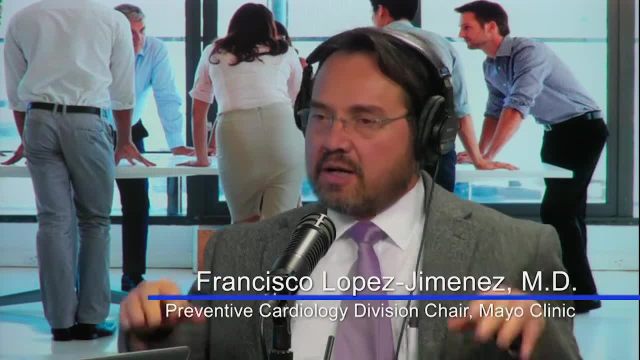 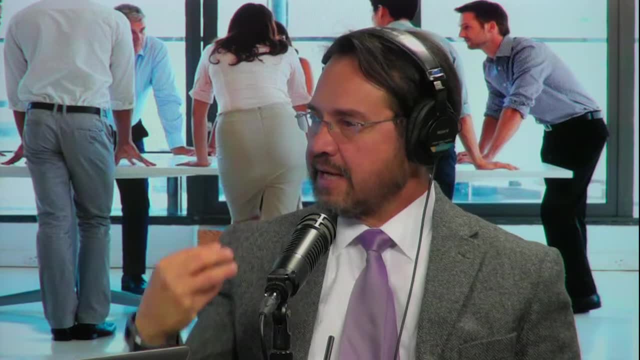 Yeah, But I'm standing most of the day at work. It's not a standing desk, It's one of those monitor holders, Oh sure, And the keyboard is the thing that goes up and down, So you can be sitting or standing. 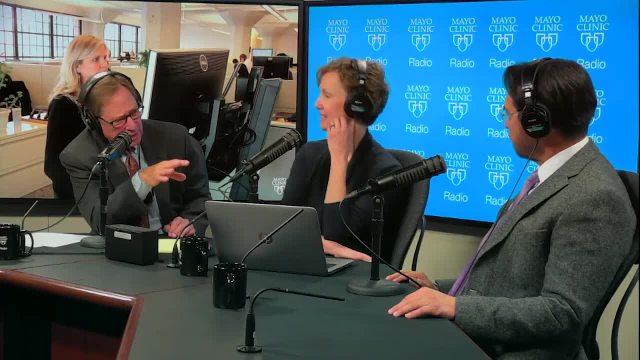 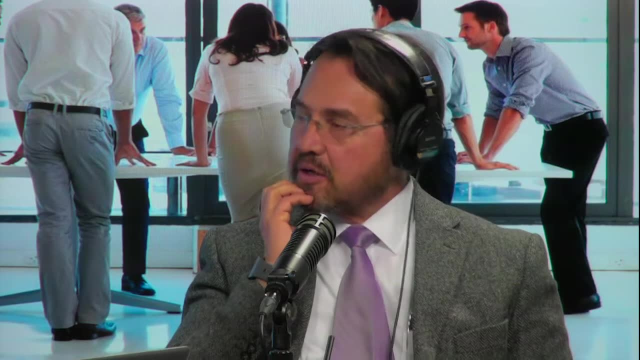 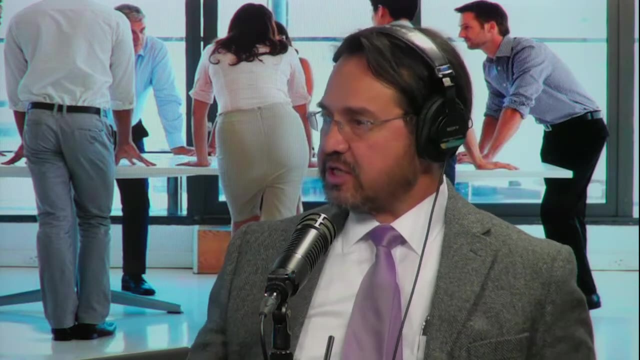 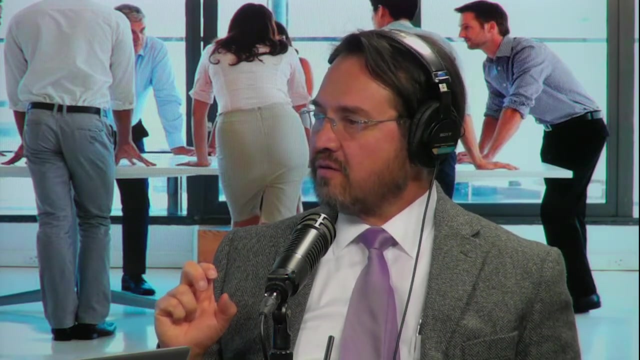 Yeah, Yeah. Is there some pretty good research to suggest that this is actually a good thing from a health standpoint? There is a lot of research showing that when you are standing, and especially when you break up the time sitting, whether it is just standing or moving around just a little bit- the metabolism of the sugar actually improves. 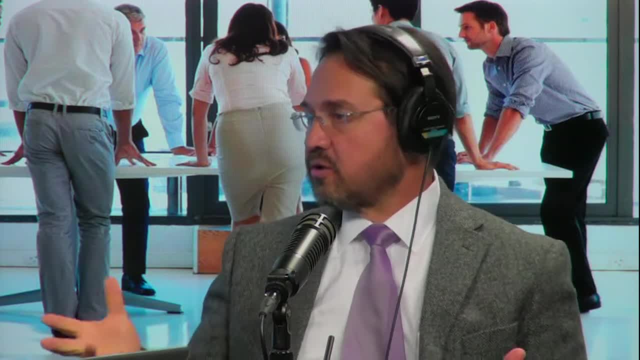 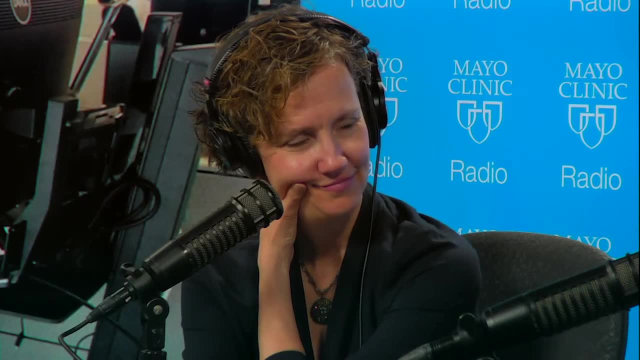 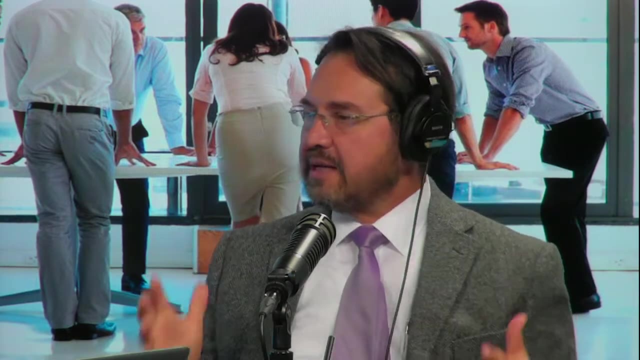 And you don't have to spend too much time based on those studies. As long as you break up those sitting times, you're good. As long as you break up those sitting times, you're good. Yeah, And at the same time, every half hour, every half an hour, you stand up and just move a little bit. 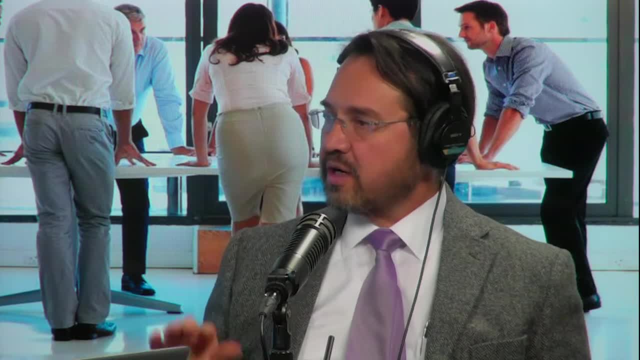 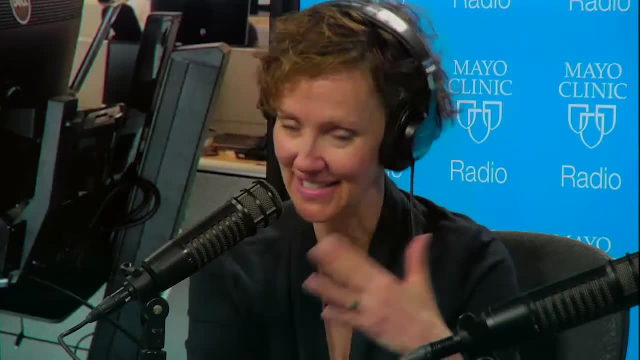 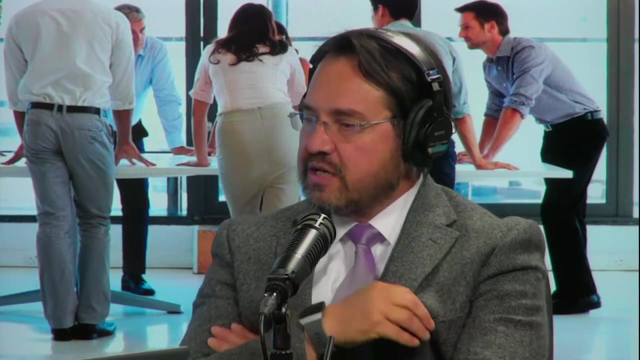 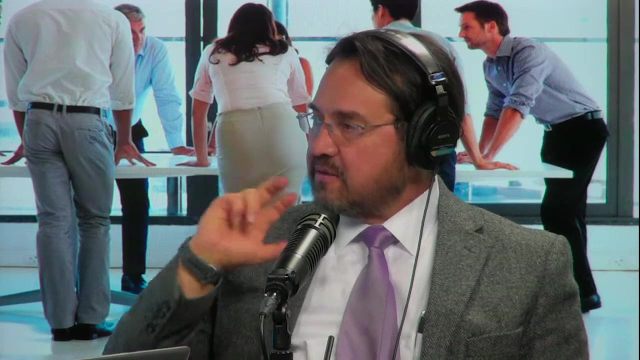 That improves the metabolism of the sugar and cholesterol and other things. What are some of the other things that your research on standing desks, or not sitting, showed you? Well, we just completed a very interesting experiment trying to see if your attention span, your typing speed, your ability to think and solve problems will change when you are standing. 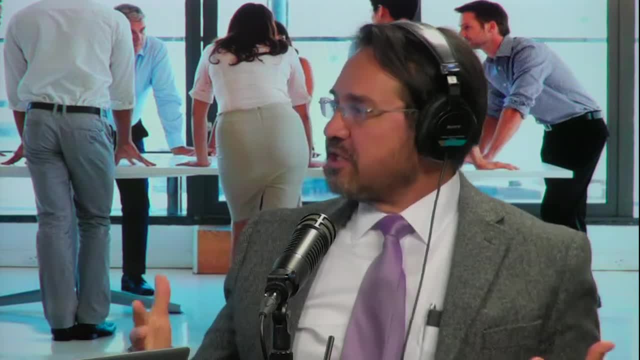 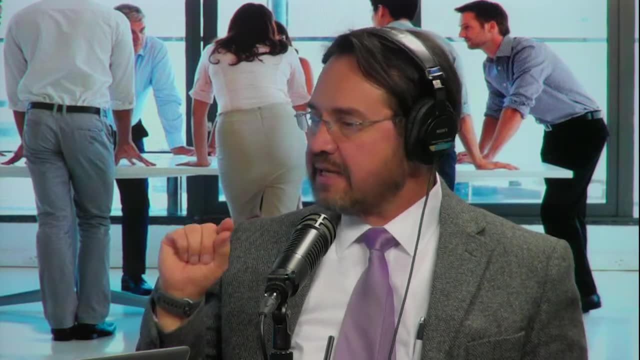 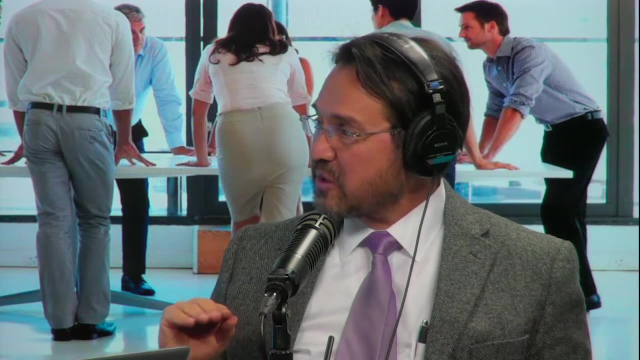 You know people say: well, you know what, when I'm standing I cannot concentrate. We tested this thing and it turns out that the concentration, typing speed and your ability to solve problems doesn't change at all And, if anything, might actually improve a little bit. 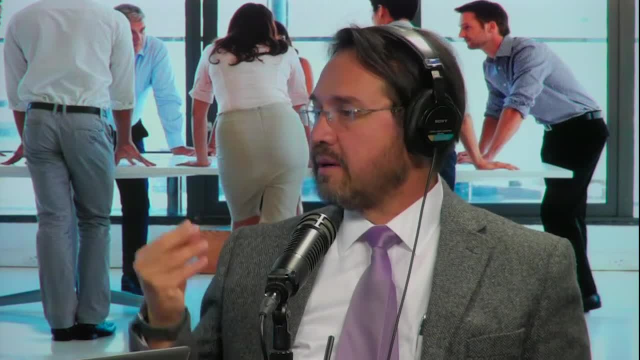 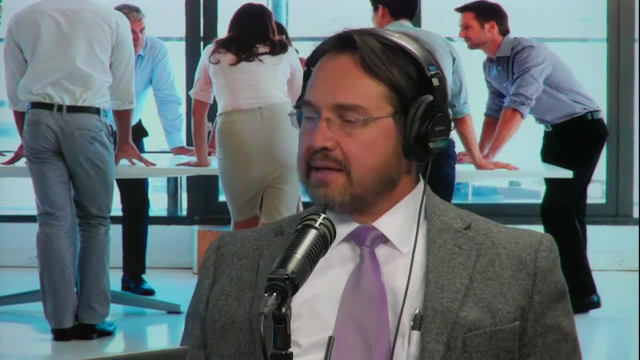 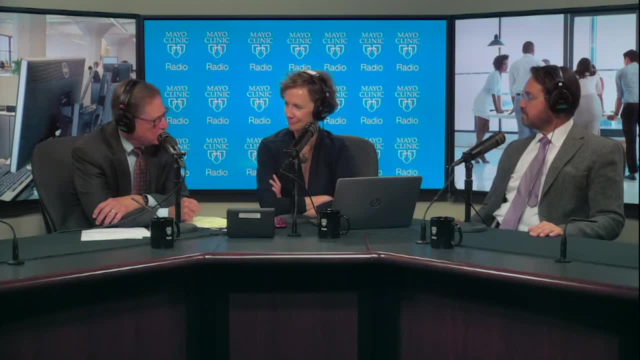 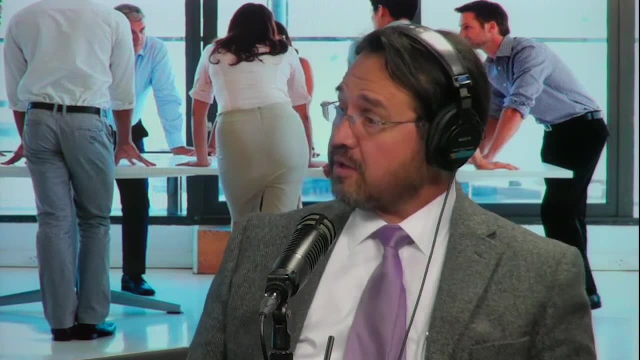 It takes about a few minutes to get used to that. Don't your legs get tired? Well, you know that's a very good point and I think it's a valid concern Whether standing for too long might affect your veins and may cause. 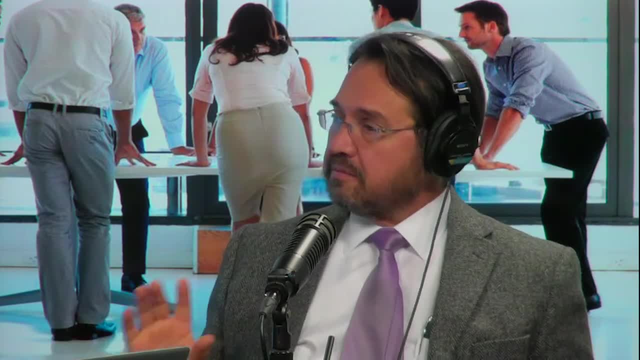 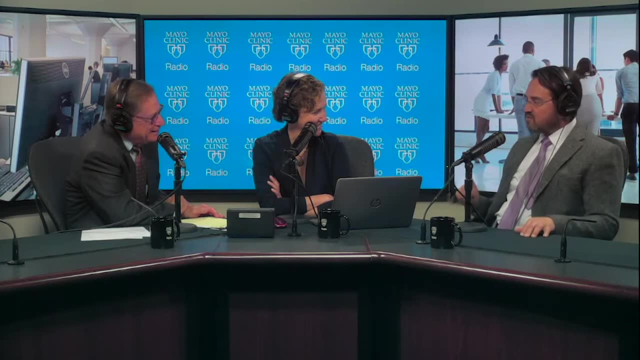 Increased incidence of varicose veins, Increased incidence of varicose veins or blood clots, or trying to find something wrong with having a stand-up, But I think that's a very important issue and I think that's why I don't believe that the solution is just standing. 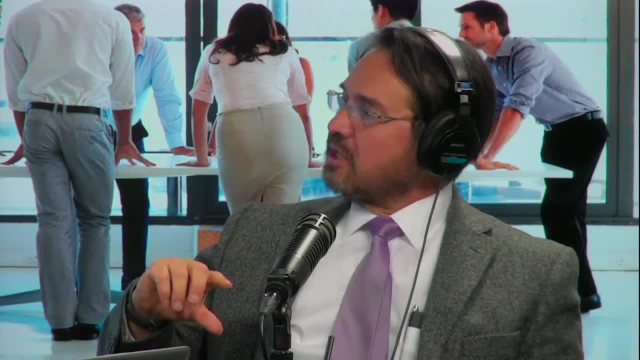 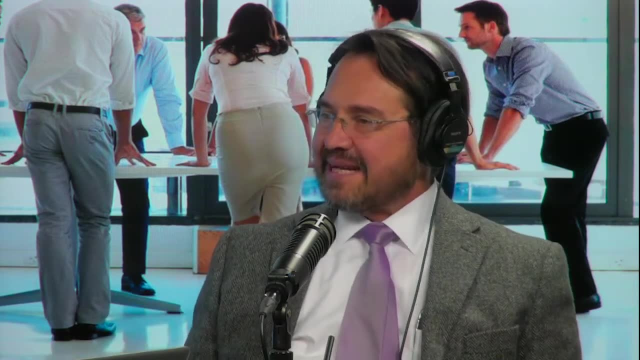 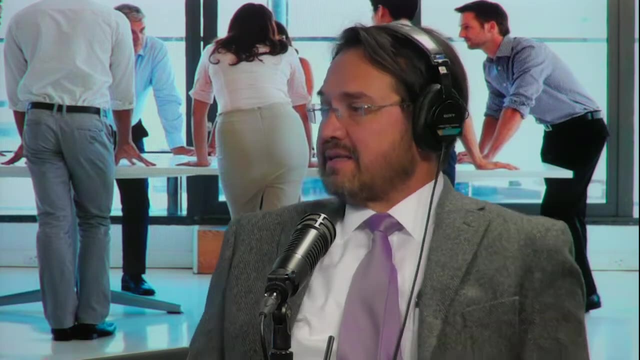 It's not sitting, which includes standing and moving. You know you don't develop blood clots when you move around, But standing alone in some people might be difficult. You might get lightheaded. Some people actually faint if you stand still for 20 minutes.